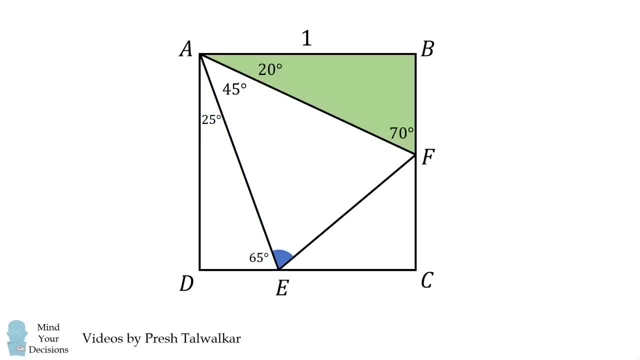 Now let's go back to triangle ABF. The trick to this problem will be to think outside the box. We will rotate this triangle 90 degrees clockwise about vertex A. We've created a congruent triangle and we'll label this vertex as F prime because it is the image of the vertex F From here. 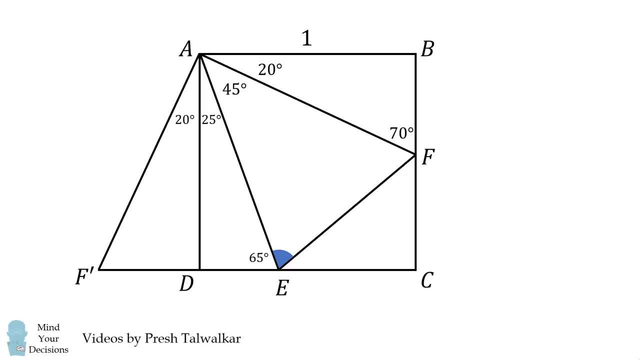 we have F prime AD is equal to 20 degrees. by construction, We then will solve that angle F prime AE will be equal to 20 degrees plus 25 degrees, which is equal to a total of 45 degrees. Now, if we want to solve this problem, we need to find the angle F prime AE. 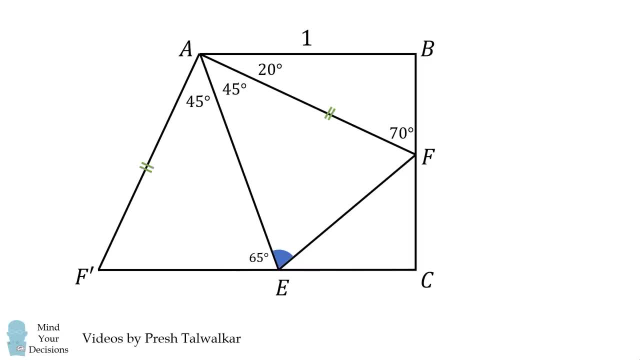 Now, if we want to solve this problem, we need to find the angle F prime. AE will be equal to 20 degrees plus 25 degrees, which is equal to a total of 45 degrees. Now we are going to consider that AF prime is equal to AF by construction. 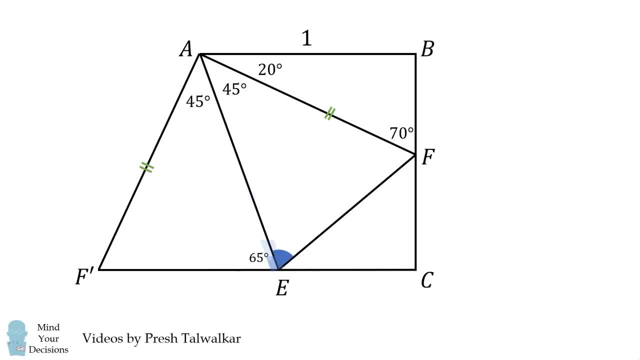 We thus have two triangles that are congruent by side angle side. Here we have one side that is equal to itself, then we have two angles that are equal to 45 degrees, and then we have two sides that are equal to each other. Therefore, these two triangles are: 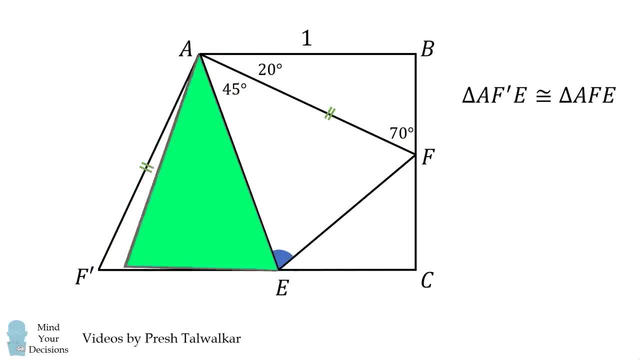 congruent. In fact they are mirror images of each other. This means angle AEF is exactly equal to angle AEF prime, and so it is equal to 65 degrees. and we are done with the first part of the question. Now let's solve for the second part of the question: What is the? 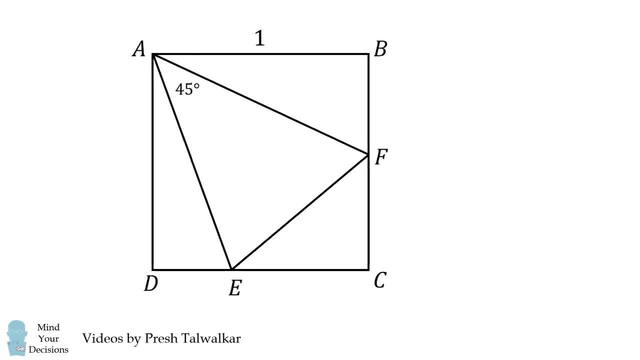 perimeter of triangle ECF. Let's consider a numerical approach. Imagine that we have a ruler and that we can measure the length of EC. Suppose we estimate it to be 0.6389.. Let's do the same thing for the other sides of CF and FE. We end up that the sum of these 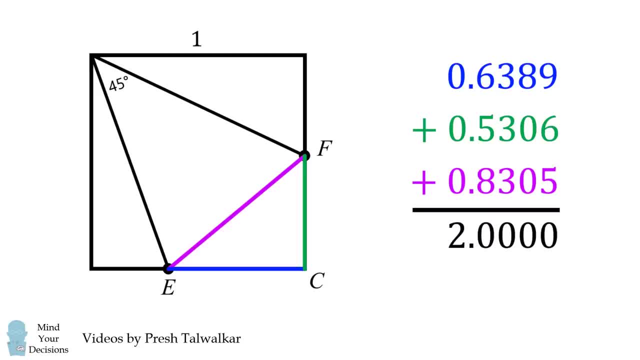 three lengths will be equal to 2.. Now what would happen if we changed the points E and F? A remarkable thing happens: No matter where we pick the points of E and F, the perimeter of this triangle will always be equal to 2 exactly.